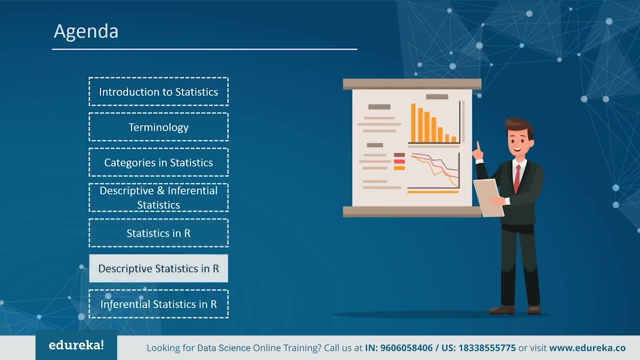 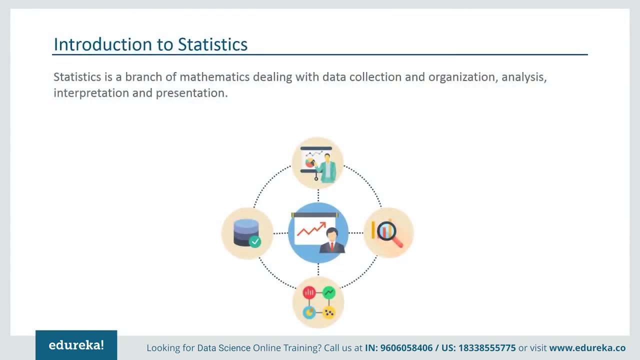 called the statistician's programming language, Then we'll be implementing descriptive statistics and inferential statistics in R. So without much ado, let's get straight into the module. So let's begin by defining the term statistics. So statistics is a mathematical science pertaining 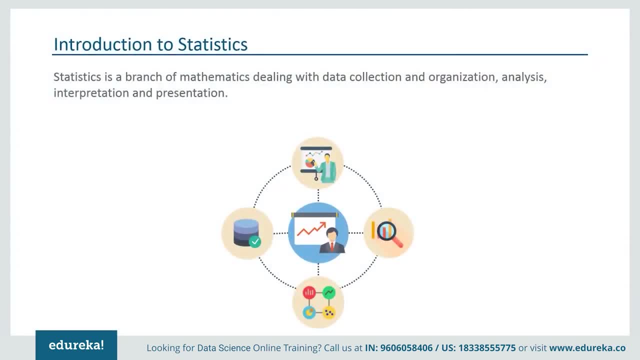 to the data collection, analysis, interpretation and presentation. It is used to process complex problems in real world so that the analysts can look for meaningful trends and changes. Analysts review data so they can reach meaningful conclusions, and several statistics, functions, principles and algorithms are implemented to analyze raw data, build statistical model. 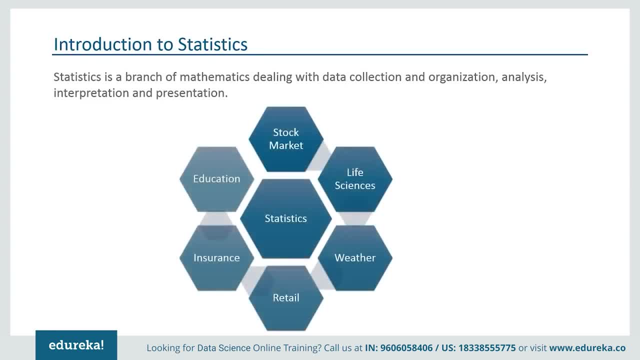 and infer or predict the results. So let's get started. So let's begin by defining the term statistics. So the field of statistics has an influence over all domains of our life. The stock market, life sciences, weather, retail, insurance and education are but to name a few With that. 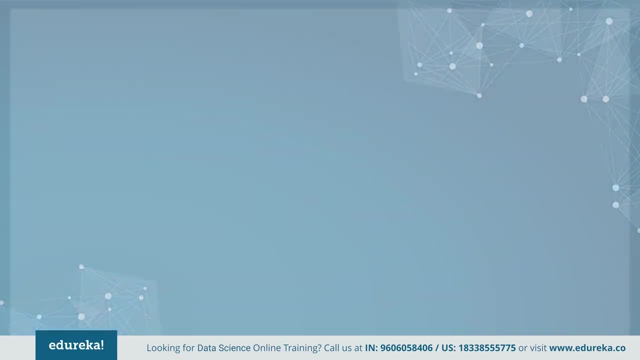 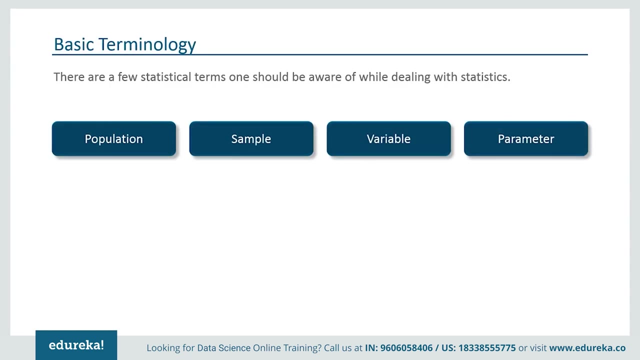 let's move on to some basic terminology regarding stats. Now, there are a few statistical terms one should be aware of while dealing with data sciences. They are namely population, sample, variable and parameter. Now, population is a set of sources which data has to be collected from. 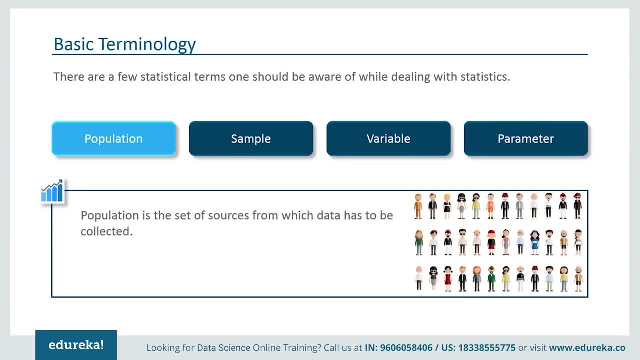 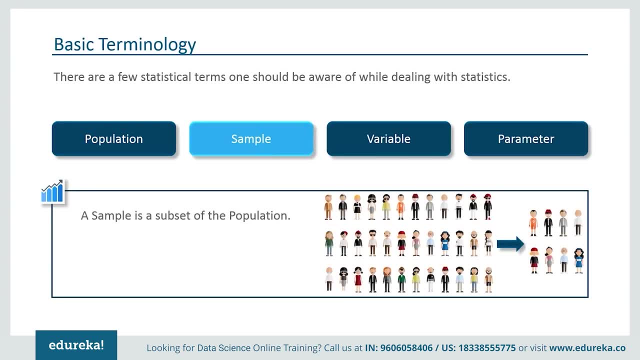 It can be a set of sources which data has to be collected from. So it can be a set of sources which data has to be collected from. So it can be a class of children, a population in a country, so on and so forth. A sample or a sample set is a subset of a wide population. You basically take 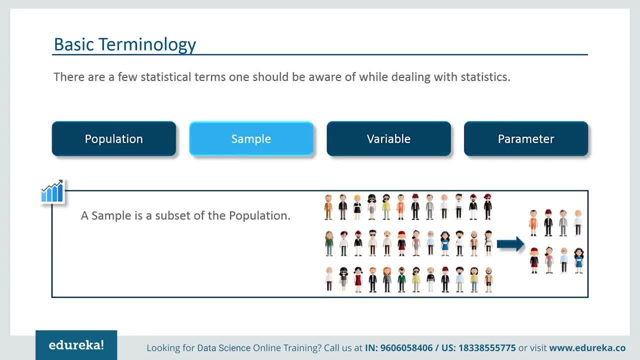 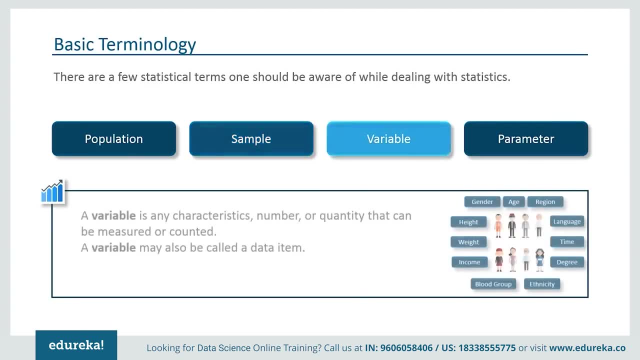 a sample set, which is a chunk of the population. You apply your statistical model to them and find out whether your conclusion holds for the entire population or no. So variable is any characteristic number or quantity that can be measured or counted When it comes to your population. 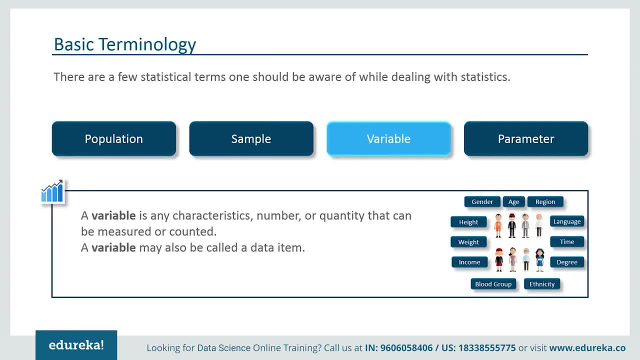 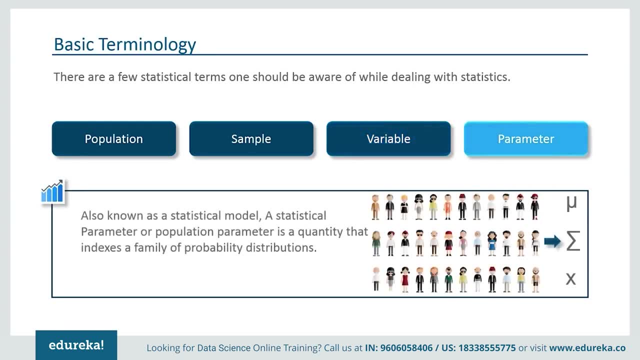 it can be their height, weight, income, blood group, ethnicity, language, time, so on and so forth. A variable is also called a data item. A parameter, which is also known as a statistical model, is a quantity that indexes a family of. 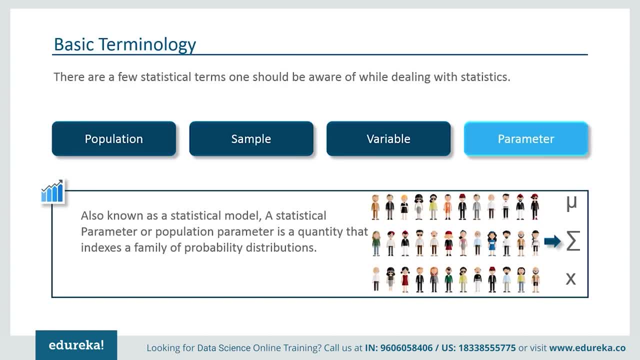 probability distributions. It can be your mean, your summation or any element of the sample set. It basically gives you a characteristic idea about a population in general. So an analysis of any event can be done in one of two ways: quantitative and qualitative. 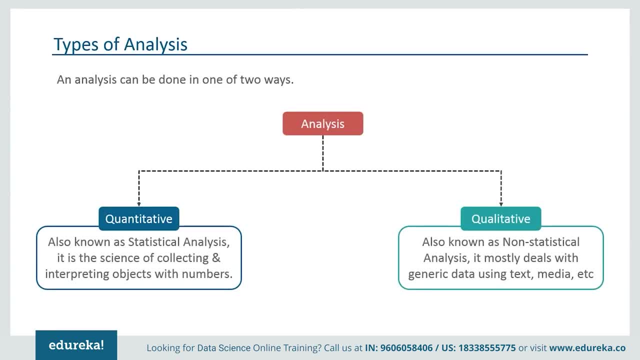 Now, quantitative analysis or the statistical analysis is the science of collecting and interpreting data with numbers and graphs to identify patterns and trends. Qualitative or non-statistical analysis gives a generic information using text, sound or other forms of media. So, for example, if I want a coffee from a coffee house, it is available to me in small 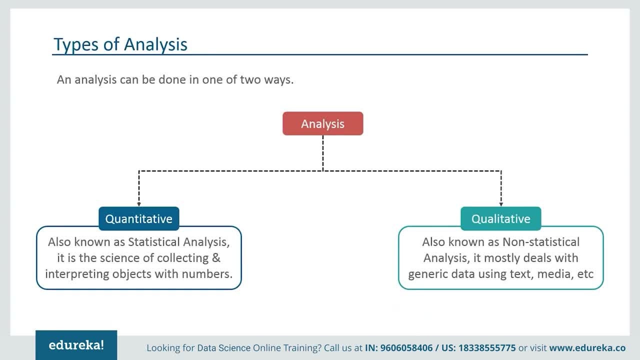 medium or large. That is qualitative analysis. There is no number. But if a store sells 50 regular coffees a week, it is a quantitative analysis, because we have a perfect number, We have a statistic, Although the purpose of both these analysis is to provide results. 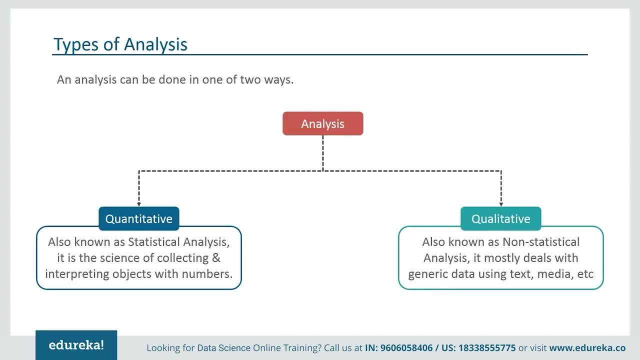 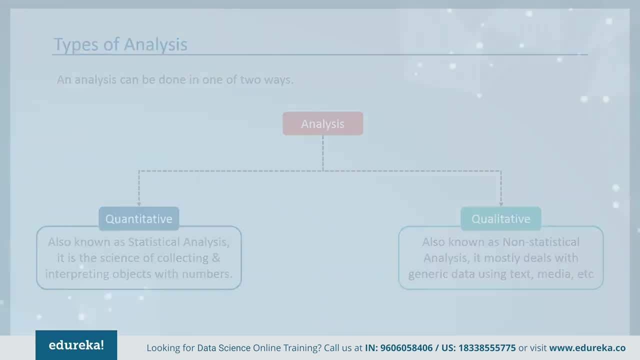 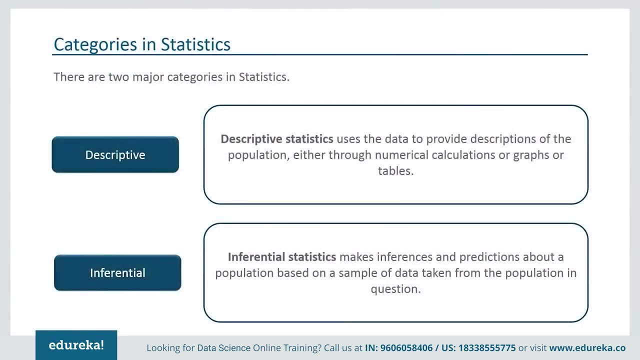 Quantitative analysis provides a clearer picture and insight, if you will. It is a characteristic that makes it crucial to analytics, And that's what we are interested in. So statistical analysis has two categories. You have your descriptive and inferential statistics. Now descriptive: 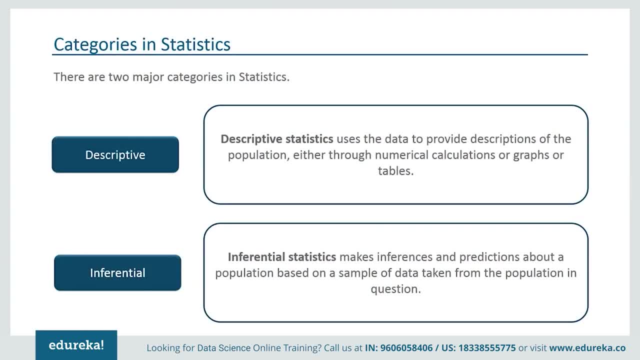 statistics, as you can see, uses the data to provide descriptions of population, either through numerical calculations or graphs or tables. Inferential statistics, on the other hand, makes inferences or predictions about a population based on a sample of data taken from population in the same question. 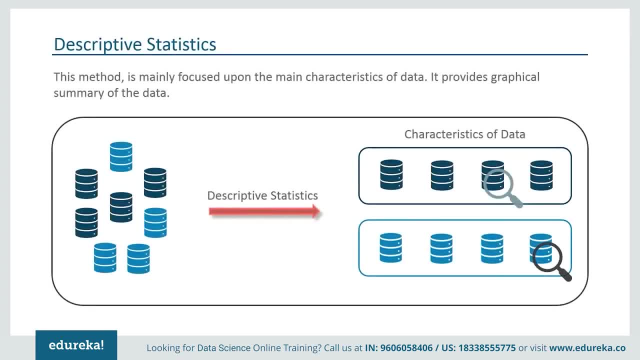 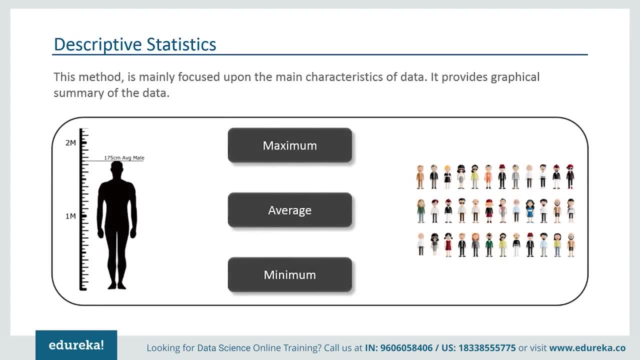 Now, descriptive statistics helps organize data and focuses on the characteristics of data providing parameters. Suppose you want to study the average height of students in a classroom. In descriptive statistics you would record the heights of all the students in the class and then you would find out the maximum, minimum and average height of the class. Inferential. 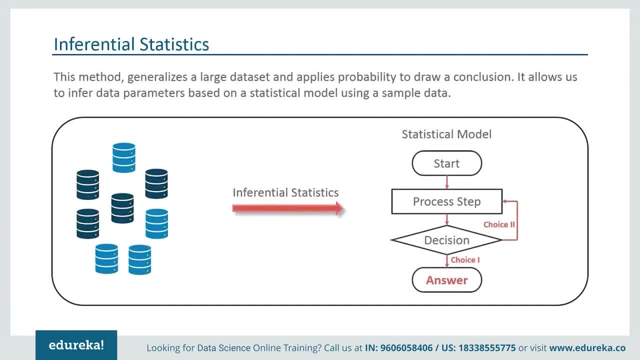 statistics, on the other hand, generalizes a large data set and applies probability to arrive at a conclusion. It allows you to infer parameters of population based on simple stats and builds models on it. So, if you take the same case of finding out the height of people, 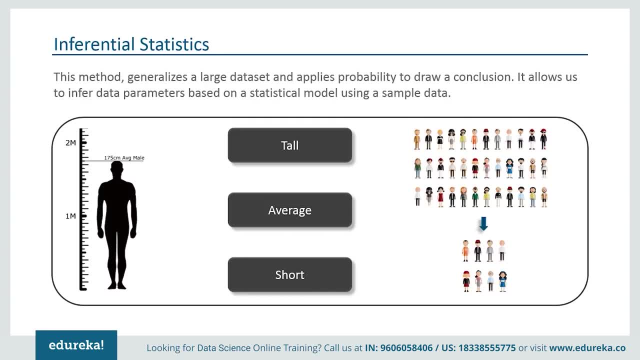 in a class in inferential statistics you will take a sample set of the class. So you have a sample set of the class which is basically a few people from the entire class. You already have had grouped the class into Tall, Average and Short And in this method you basically 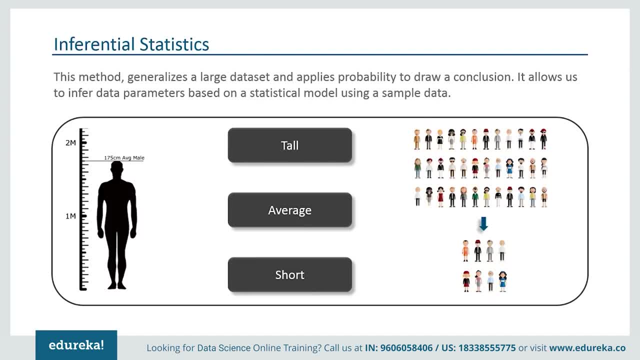 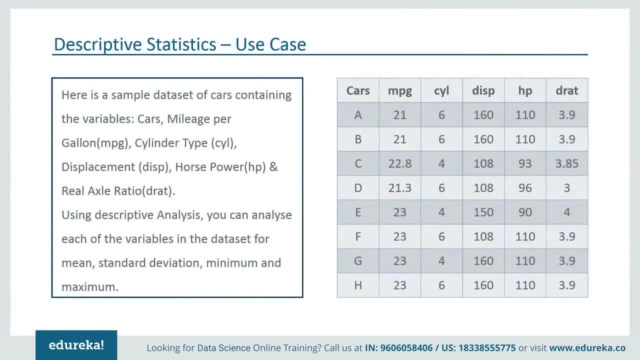 build a statistical model and expand it for the entire population in the class. Now let's talk a little bit about descriptive analysis. So we try to represent the data in forms of graphs and histograms and line plots etc. But the data represented is based. 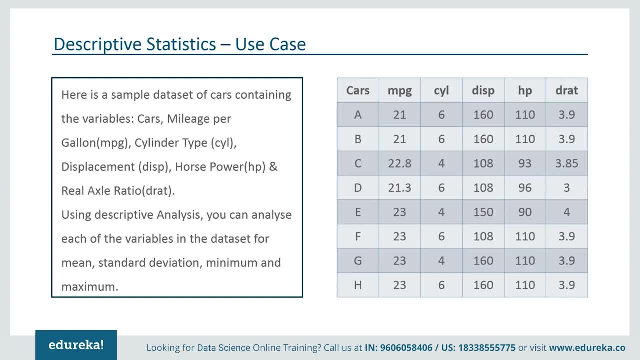 around some kind of central tendency Means that the particular graph represents distribution. the mean or measures of spread depends on what you want from your graph. so for that we have a few measures in statistics. let me give you an example for better understanding. so here is a sample set of cars containing variables. 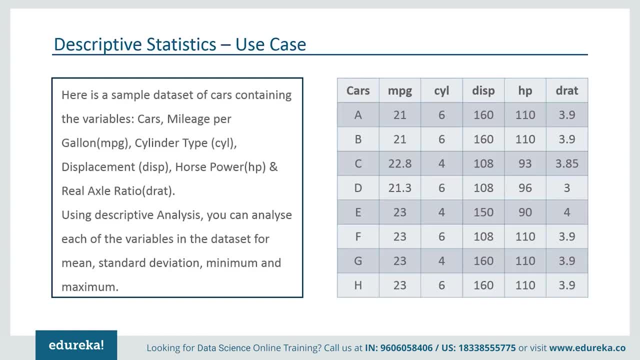 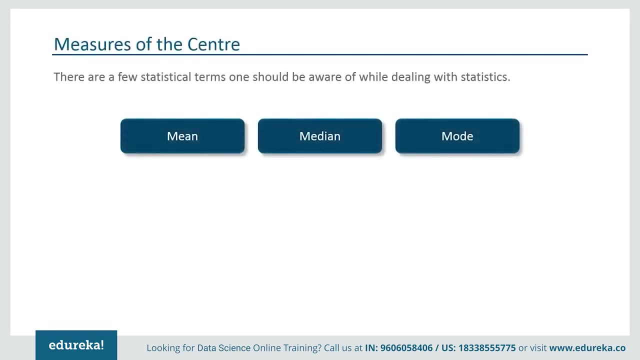 cars: mileage per gallon, which is mpg- cylinder type, displacement, horsepower and real axle ratio. using descriptive analysis, you can analyze each of the variables in the data set for mean, standard deviation, minimum and maximum of the range. now, first of all, we're going to discuss a few measures of the 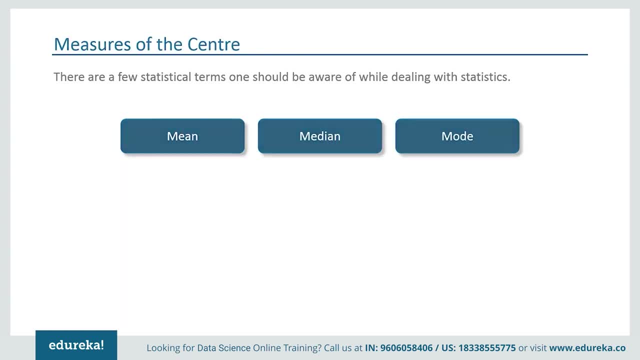 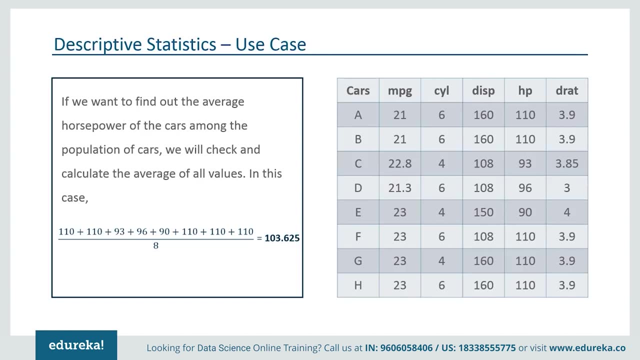 center. these are also called measures of central tendency. now, if we want to find out the average of horsepower of all the cars among the population of cars, we will check and calculate the average of all values. in this case, we'll take the sum of all these values and divide them by the number of cars we have. we get an. 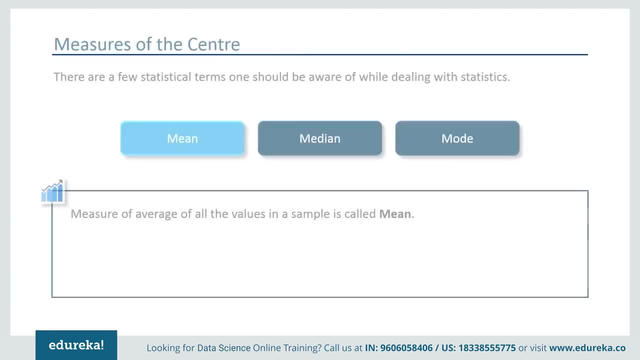 answer of 103.625. so this is basically the mean of the horsepower, which is the measure of average of all values in a sample. so mean gives you an average of an entire data set. suppose I say the average marks in the 10th board exams of students of a certain school is: 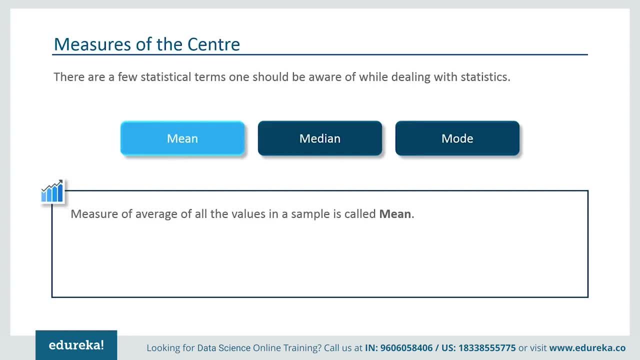 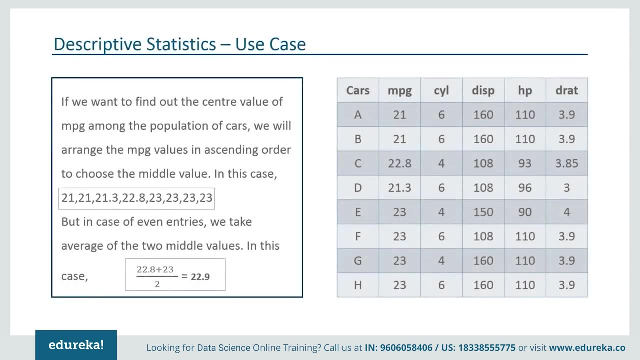 85%, then that particular data will give us a notion that the whole school, that at an average, each student scores about 85% and the central tendency of that school is to usually perform well. next we have median. if you want to find out the central value of mpg amongst the population of cars. 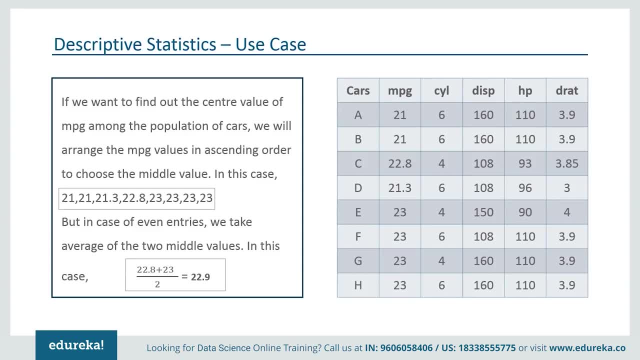 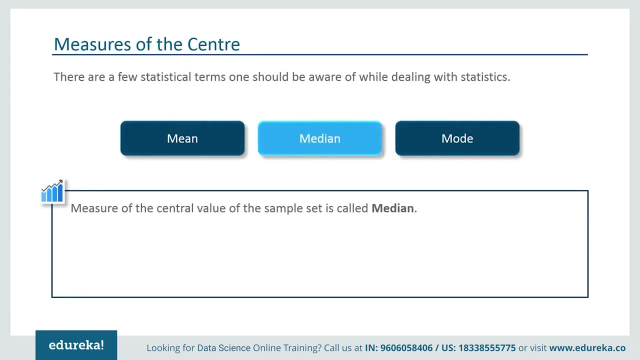 we have to arrange all values in either ascending or descending order and choose the middle value. in this case, since we have an even number of values, which is eight values, we take the average of the two middle values. in this case it is 22.9. therefore, the measure of the central value of a sample set is called 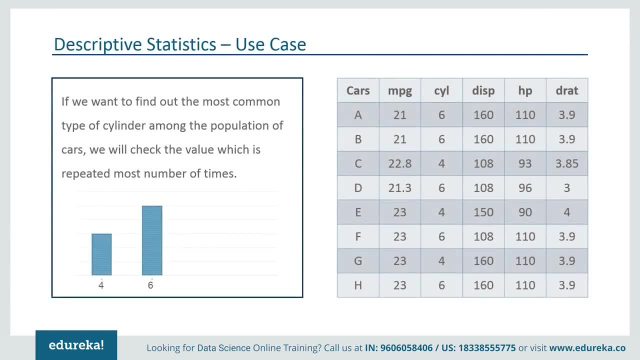 a median. next, if we want to find out our most common type of cylinder amongst the population of cars, we will check the value which is repeated most number of times. here we can see the cylinders come in two values: one is four and one is six. so the most recurring value, according to the graph, as we can see, is six, so that 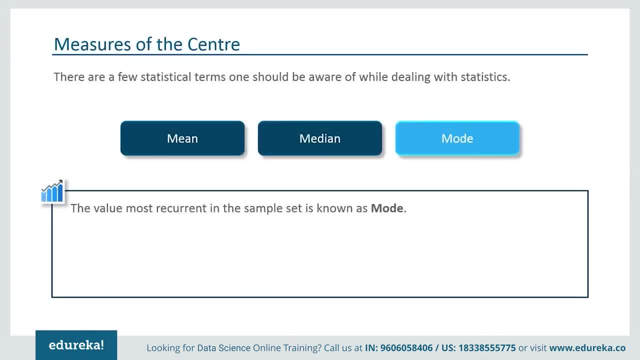 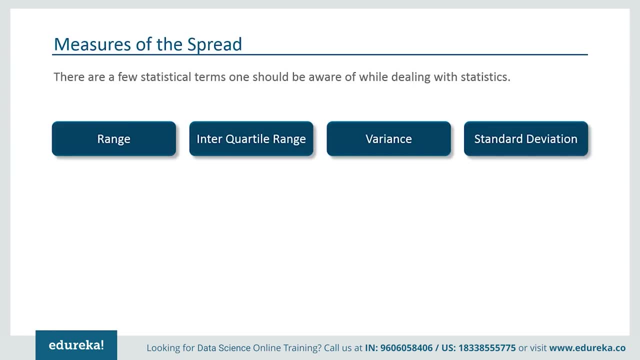 is our mode, which is our most recurrent value in the sample set. now, like the measures of the center, we also have measures of the spread. this comprises of the range, interquartile range, variance and standard deviation. so range is basically is the value between the maximum and the minimum. you can see the 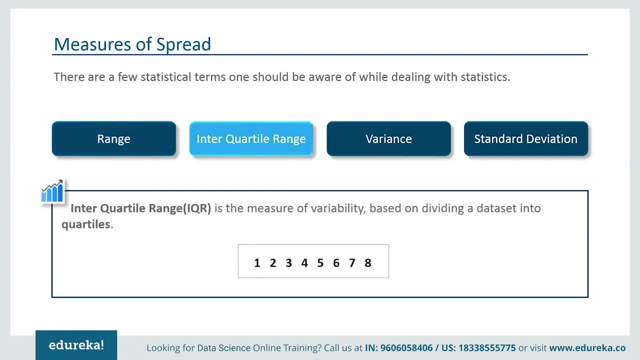 formula is as given, similar to the range, there's something called the interquartile range. for this you'll have to know what is a quartile. now, as you can see, we have a sample set from numbers one to eight. so basically, the purpose of quartile serves is to divide your entire data set into. 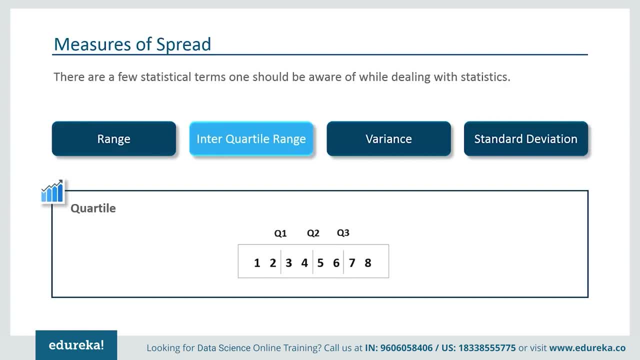 four quarters. so you have your q1, q2 and q3, which are the three quartiles. they are your division points and you can determine their values like. so this is your q1, your q2 and your q3, as you can see, basically you take the division, the number on either side of it. 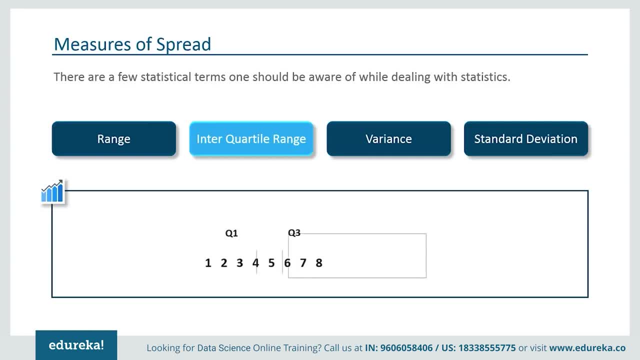 and you take an average of both those numbers and the difference between your q1 and q3 is basically your interquartile range. next we have variance. a variance basically describes how much a random variable differs from its expected value. it basically entails computing squares of deviation. I'll 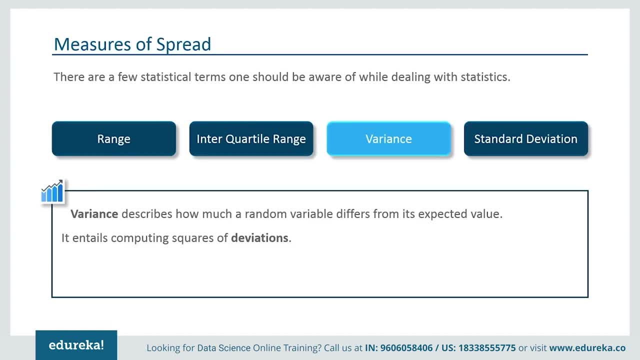 explain to you in just a little while now. there are a few crucial terms which fall under this. the first one is deviation, which is basically the difference between each element from the mean. you can see the formula is given below. your population variance is the average of squared deviations and you have your sample. 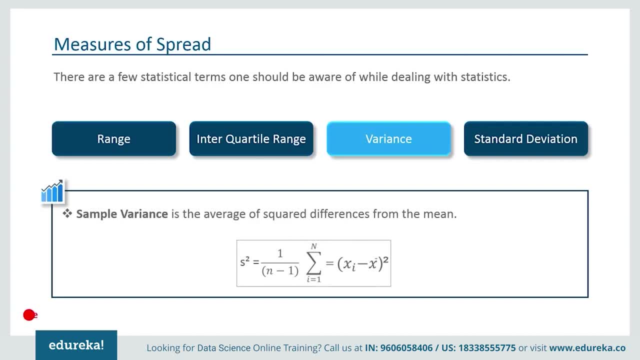 variance, which is the average of squared differences from the mean. now, as you can see, all of these terms revolve around the mean value. this basically give you an idea of how much an element varies or deviates from your mean value. now we have the standard deviation, which is the final measure of spread is the measure. 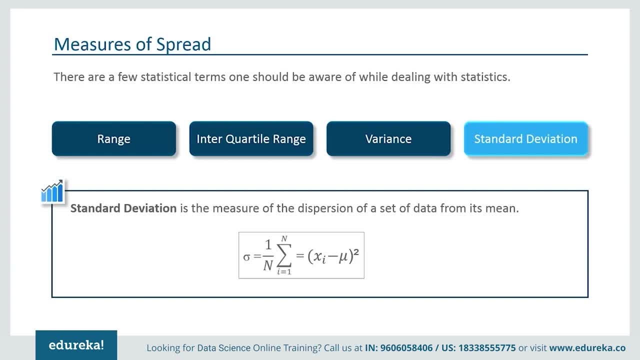 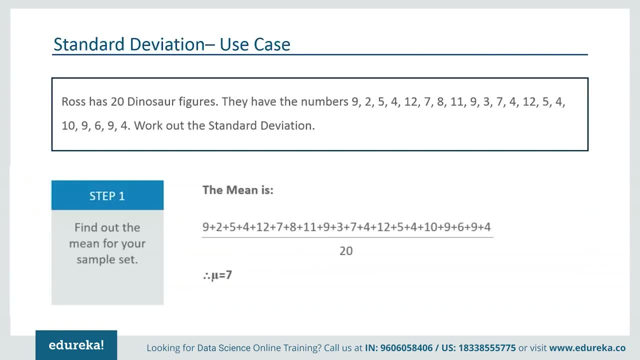 of dispersion of a set of data from its mean. since it is such an important term in statistics, we are going to find out how to take out the standard deviation. for that we have an example, so this is basically how you should calculate a standard deviation. so let's read our problem statement: Ross has 20 dinosaur. 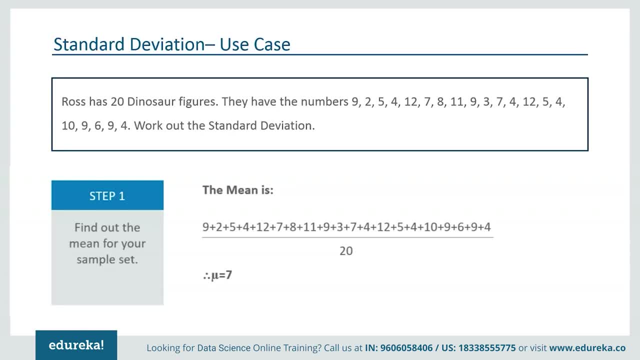 figures. they have the numbers 9 to 5 for twelve, seven, eight, eleven, nine, three, seven, four, twelve, five, four, ten, nine, six, nine and four on them. wow, that was a mouthful. so what we have to do is we have to work out our standard deviation. 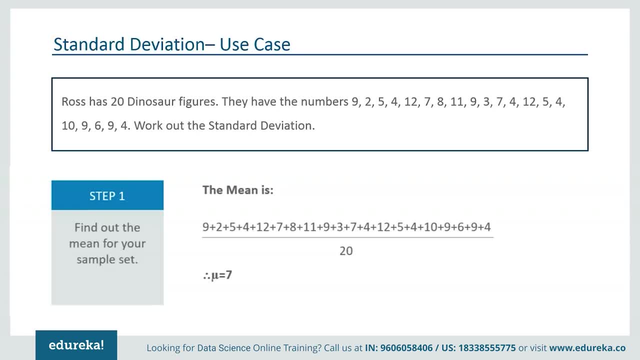 so step one to it is to find out the mean. the mean here is 7. as you can see, average of all the numbers divided by 20 it's 7. next, for each number, you have to subtract the mean and square the result. now, why are we squaring the results is basically to nullify any sign difference that. 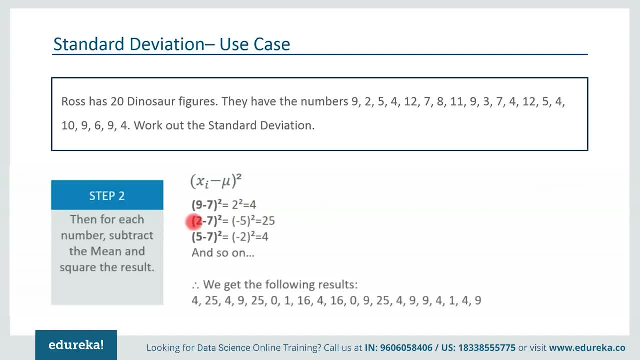 comes in our results. as you can see, in the second row we have 2 minus 7 and the result is going to be minus 5. in such a case, if we square it, we can bring it to a positive sign. here you can see we have 25. same goes for the third number. next we work out the means of those squared differences. 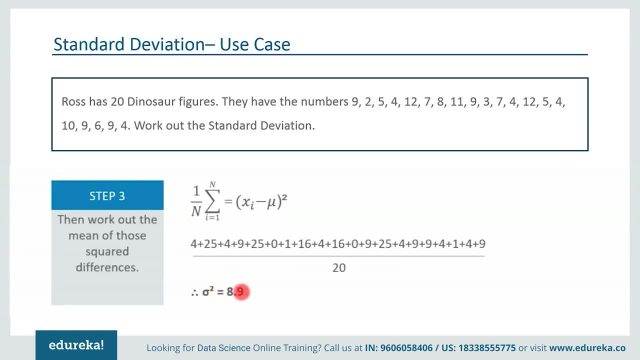 and we get a value called sigma square. if you remember, this is also the formula for the population variance. now, why population variance is the formula for the population variance? so, if you remember, this is also the formula for population variance- is because there's something called the degree of freedom, which is a topic for 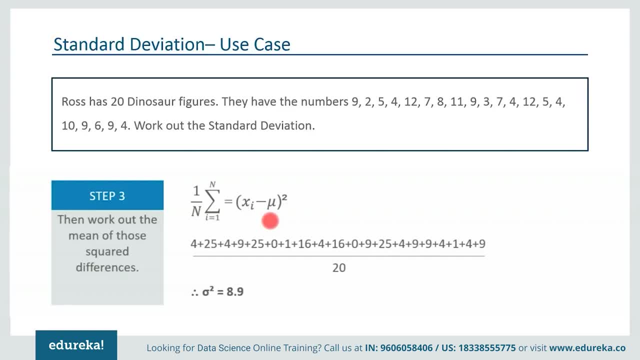 another day. but all you must know is the degree of freedom we need to subtract from the samples, and that is why we take out this value. next, if we take a square root of sigma square, we get our sigma, which is basically our standard deviation. our standard deviation here is 2.983. now that we've 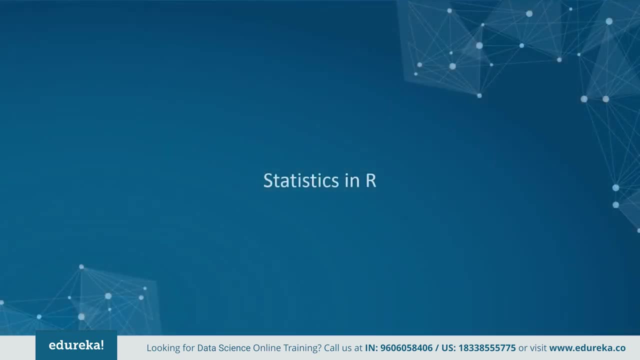 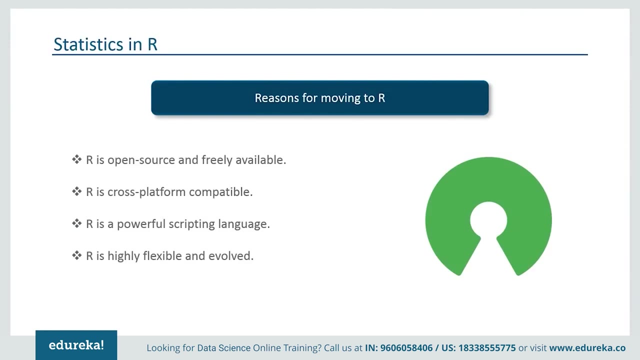 seen the math that goes into it. let's try to work it out in our now. there are quite a few reasons to why the world is moving towards r. a couple of them are enlisted here. now r is open source and freely available. it is absolutely free and there are no hidden costs, unlike sas or matlab. you can freely. 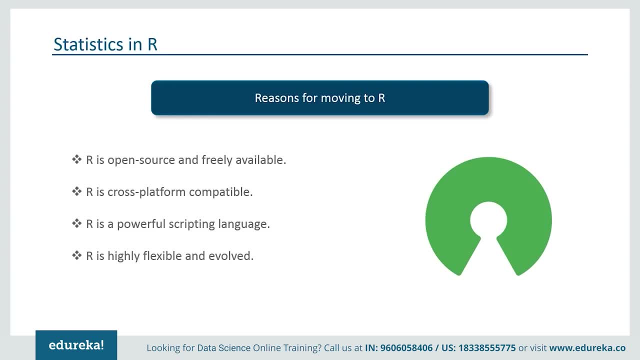 install, use, update, clone, modify, redistribute and resell r. this saves a lot of the company's money, but it also allows for easy upgrades, which is useful for statistical programming languages. now r is used across all platforms, so r can be run on windows and windows app and it can be run on 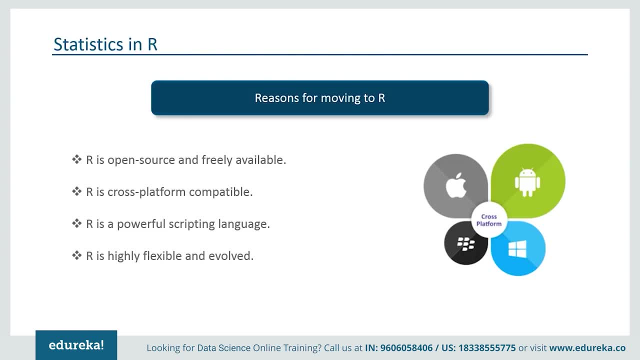 mac os and linux. it can also import data from microsoft: excel, microsoft access, mysql, oracle and other programs. next, r is a powerful scripting language. as such, r can handle large, complex data sets. r is also the best language to use for heavy resource intensive simulations, and it can. 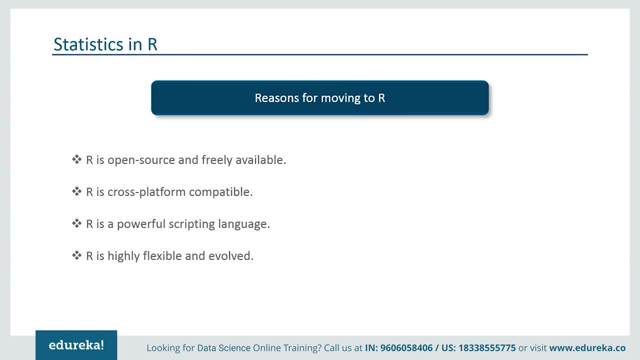 be used for high performance computer clusters. finally, r is highly flexible and evolved. many new developments in statistics first appear as r packages now. because of these reasons, r has a huge, vibrant community and resource bank, with a global community of passionate users who regularly interact on discussion forums and attend conferences. 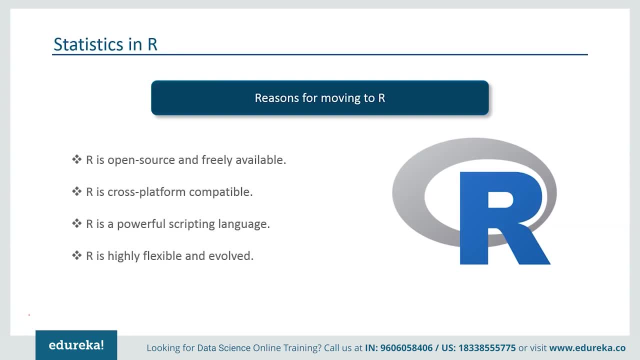 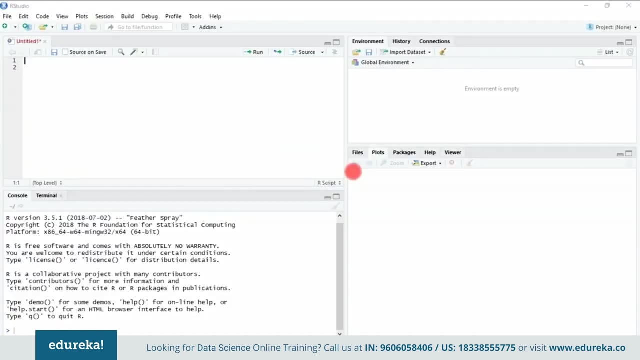 in addition, about 2000 free libraries are available for our unlimited use, covering statistical areas of finance, cluster analysis, high performance computing and much more. now, enough chit chat, let's get some work done. so our studio now. r is a programming language. we use it to do statistical and quantitative analysis. so this is r studio on. 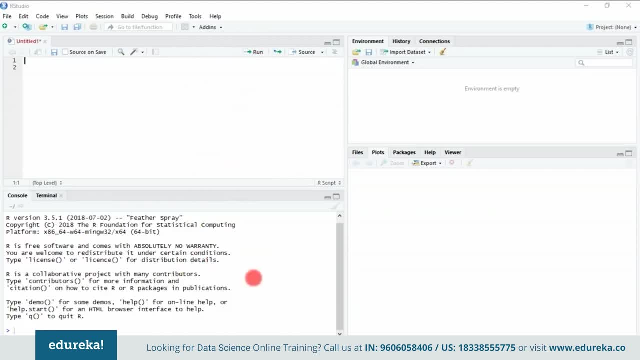 the top left is where we write the code. beneath it is the console. on the top right we have our environment, where we see any objects that we create, and at its bottom we see where our plots are. now let's run some descriptive statistics code here. like we saw how we take out the mean. 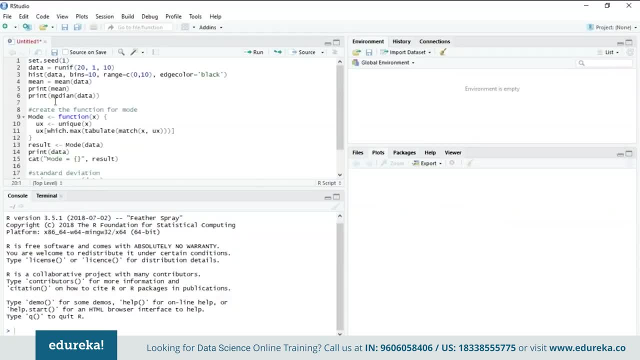 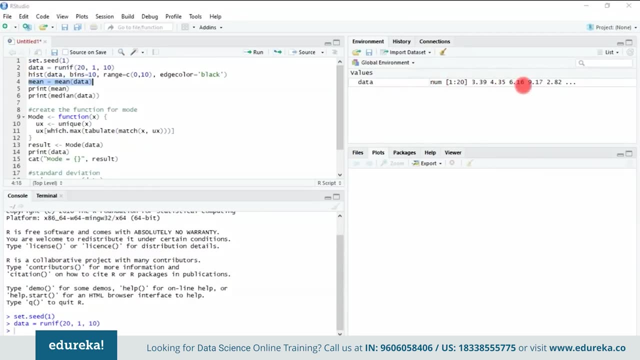 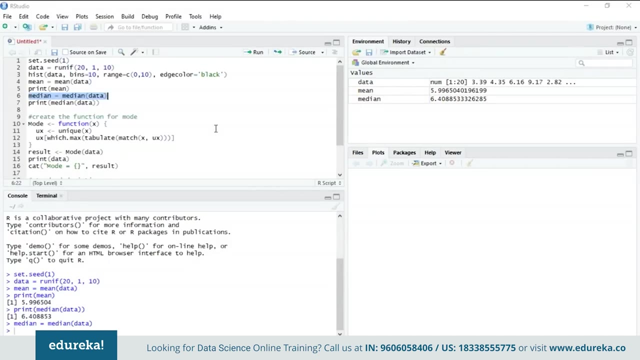 median and mod. i have some code here for mean and median. we have our direct functions here. you can see this is our data right here. we can find our median here as well. in order to get mode value, we can define our own function in our. we can just get a unique set of values and get the mode for the data set. 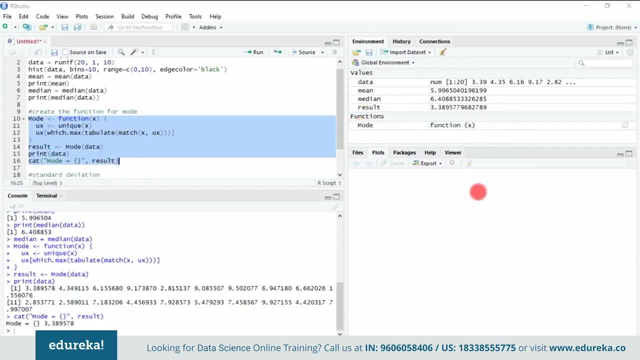 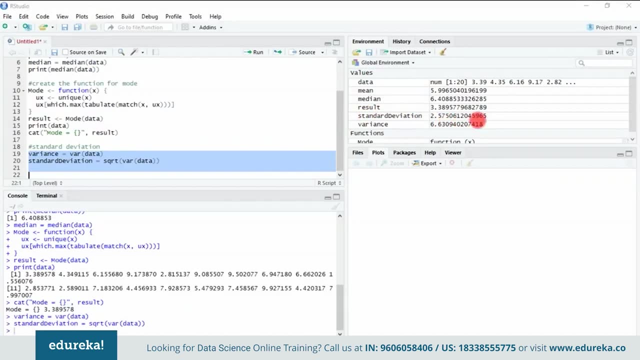 as we can see, the mode appears right here, the function. we have printed out the mode. now for standard deviation, we have to take the square root of variance. as you can see, we have created an object called variance here and the standard deviation here. we take the square root and it. 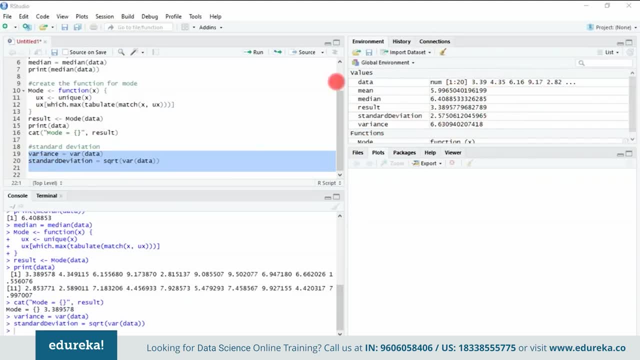 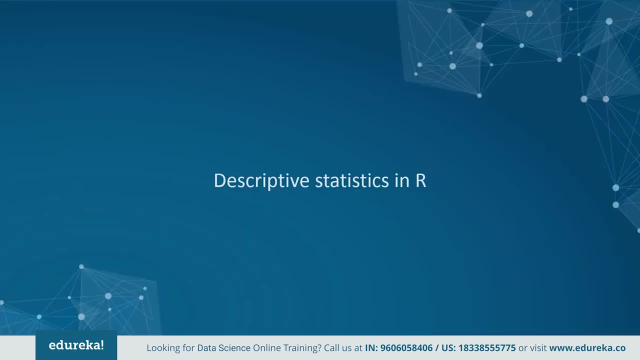 appears right here with all the other objects that we've created now, and we can also create a histogram. all we have to do is use the function hist and pass on the parameters. here you see, we have the histogram of our data right here now. so far, you've learnt about descriptive statistics. 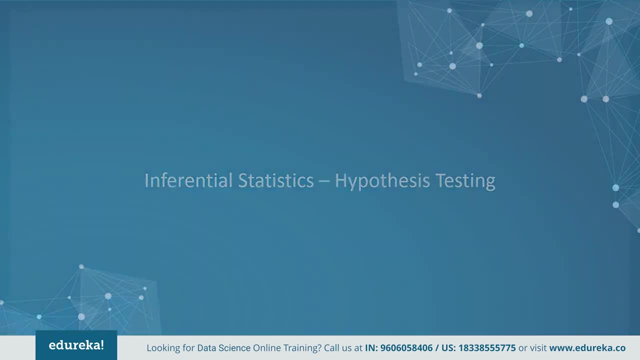 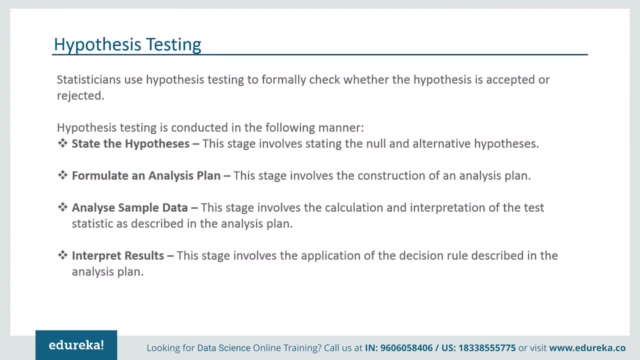 let's talk a little bit about inferential statistics. so hypothesis testing is an inferential statistical technique to determine whether there is enough evidence in a data sample to infer that a certain condition holds true for an entire population or not. to understand the characteristics of a general population, we take a random sample and analyze the properties of the 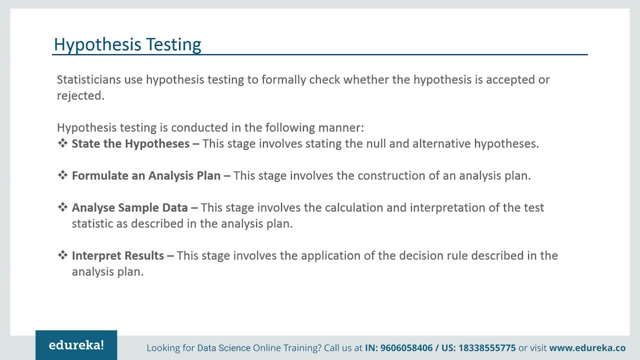 sample, we test whether or not the identified conclusion represents the population accurately or not and finally, we interpret their results. whether or not to accept the hypothesis or not depends on the percentage value that we get from the hypothesis. so let's try to understand this using a general example. now consider four boys. let's 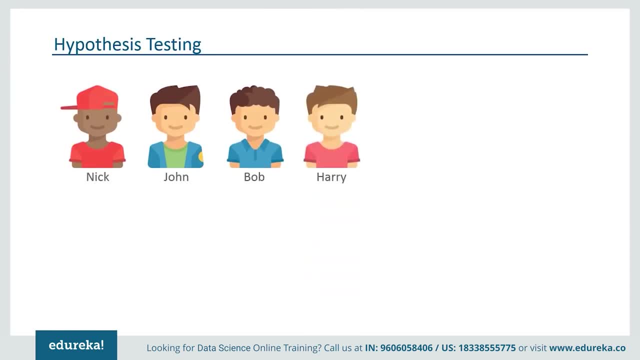 call them Nick, John, Bob and Harry. now all these four boys have to take turns in cleaning the class. now John comes up with this genius idea of writing their names on chips and putting them in a glass bowl. every day they would pick up a name from the bowl and 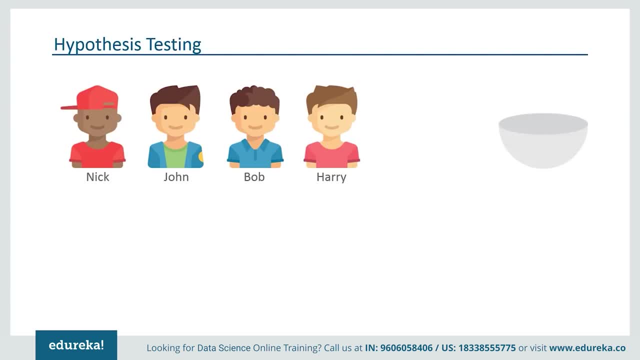 that person has to clean the class. now it has been three days and everybody's name has come up except John's. now, assuming that this event is completely random and free of bias, what is the probability of John not cheating now if we give him the benefit of doubt? let's consider if John is not picked for a day. 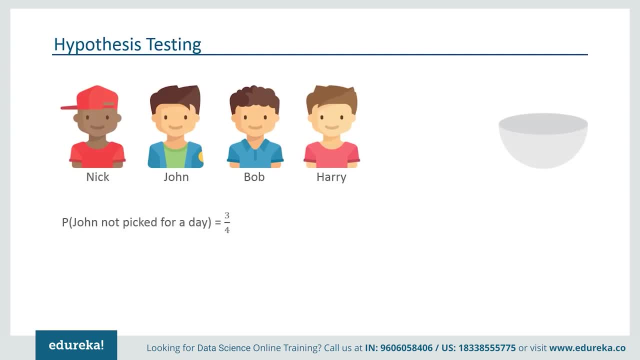 the probability is fairly high. we have a three by four probability, which is 75%. now, if John is not picked for three days in a row, the probability drops down to 0.42 approximately, which is also 42%. now let's take a situation where John 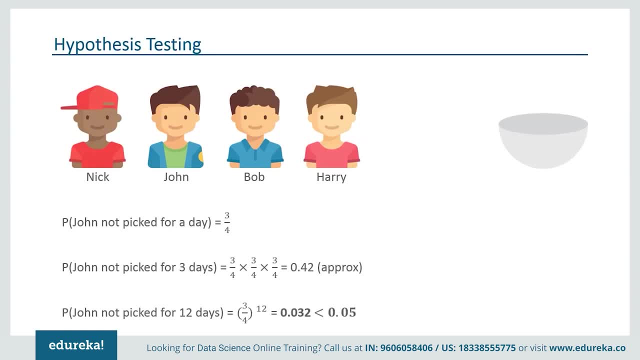 is not picked for many, many days in a row, let's say twelve days in a row, the probability goes down to 0.032, which is also 3.2 percent. and this is what statisticians do, right: they define thresholds and say hey if the 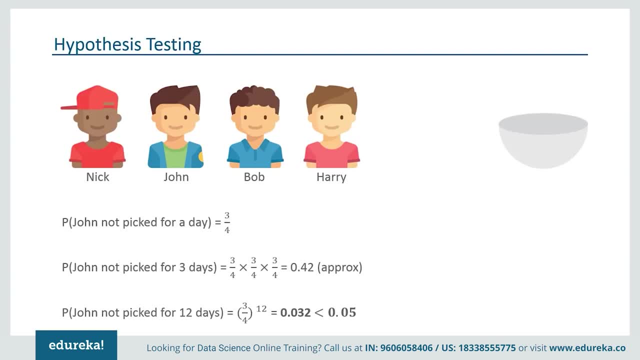 probability of this happening is more than 5%, then I'll consider it happening by chance. If it is less, then, given this example, John is surely cheating in some way or the other. And this number will keep dropping more and more if you increase the number of days. 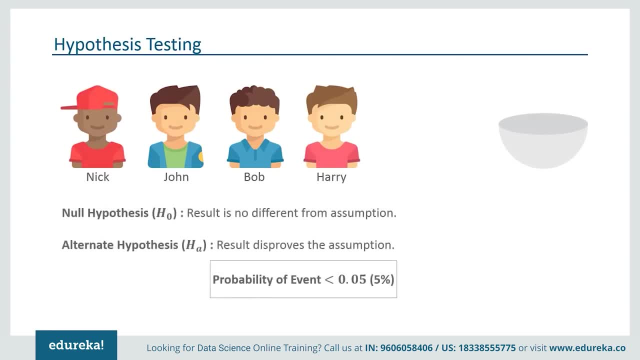 So this gives rise to something called null hypothesis. If your result is no different from the assumption, it is called null hypothesis. An alternate hypothesis is a result that disapproves the assumption. If a probability of an event is less than 5%, it is most probably a biased event. 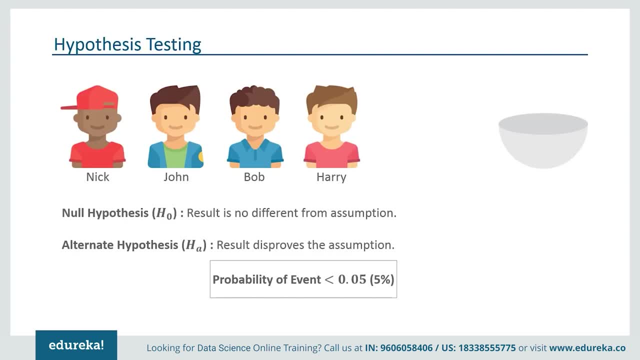 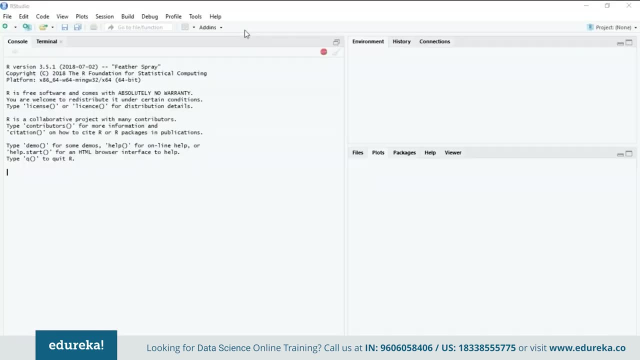 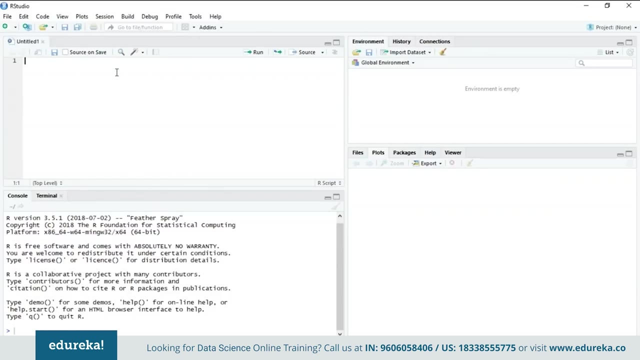 Hence the alternate hypothesis. So I'll be using a data set and showing this to you in R. Okay, let's clear this out. Let's get our R script. Okay, so I'll be using a data set called gapminder so you can download it to your computers and use it simultaneously. 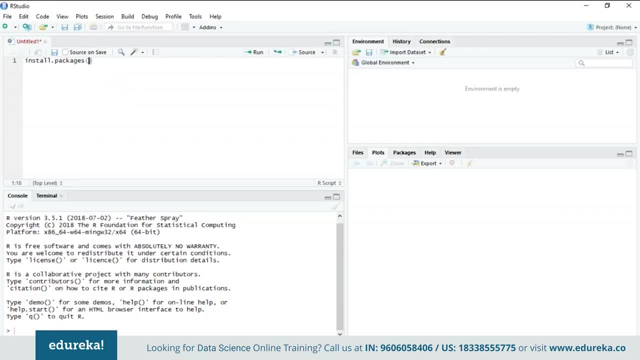 To install the gapminder data set you'll have to use install package gapminder and put it in inverted commas. Now you don't have to install it every time you use it, but you've got to call it. so we use the library function gapminder, no inverted quotes this time. 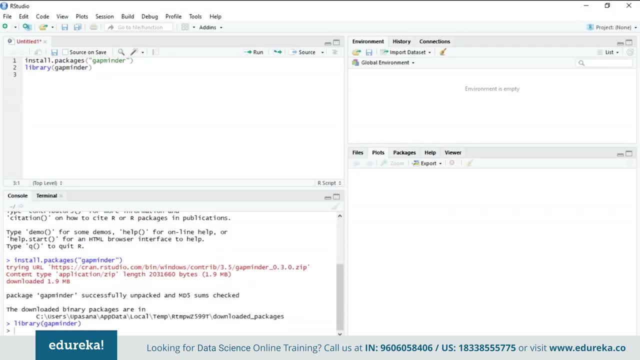 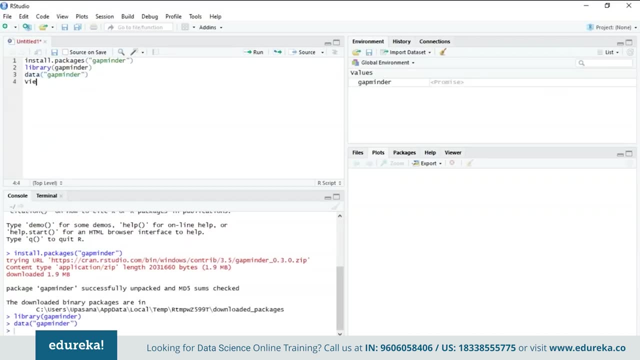 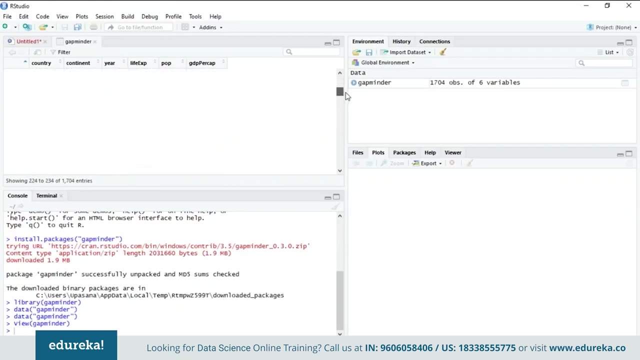 Now you can, but don't have to use the data which makes it visible on the right in your environment to view the functions. So yeah, now you can see your entire data set. So you can use the same data set. So yeah, now you can see your entire data set. 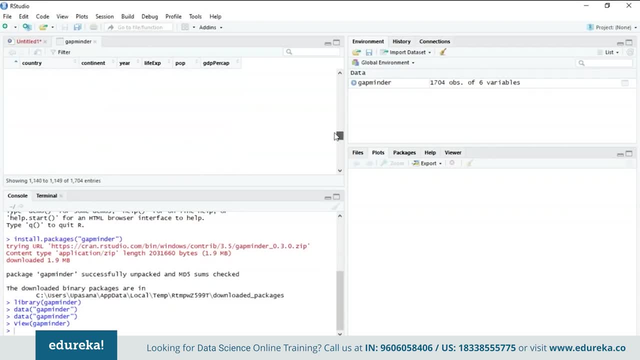 To do all the descriptive statistic codes that we've run till now. but here we are going to use this for our inferential statistic codes, which is basically for hypotheses testing. You can see country, continent, year, life expectancy, population and GDP per capita. 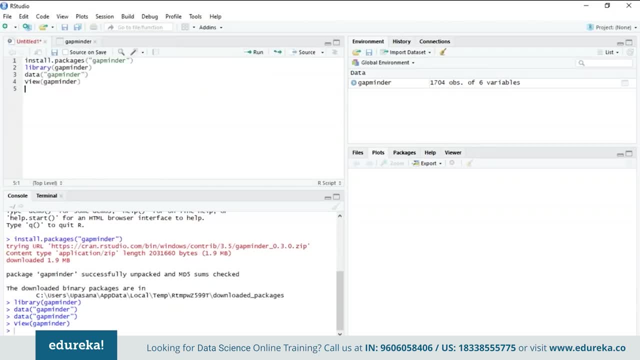 These are the columns or variables that we have here. Okay, so we've got a data set and we might want to start by doing some manipulation, And to do that we need to use a dplyr package. So dplyr package is one of those. 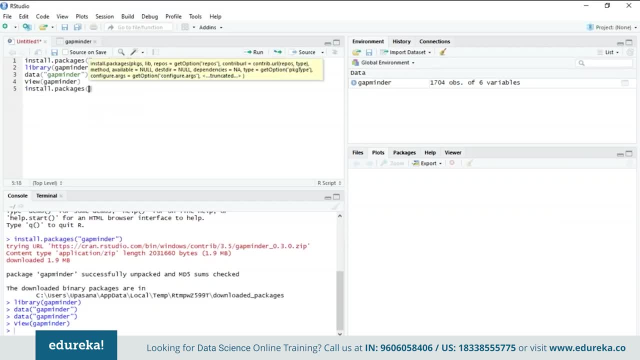 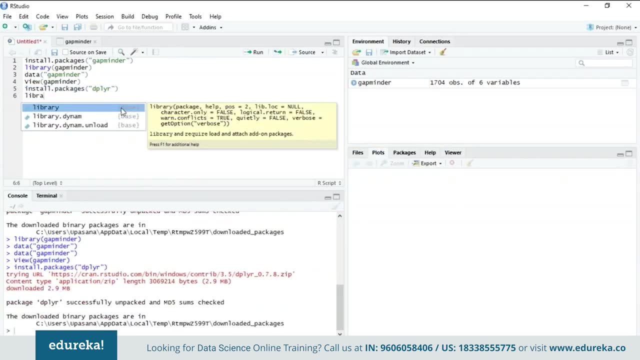 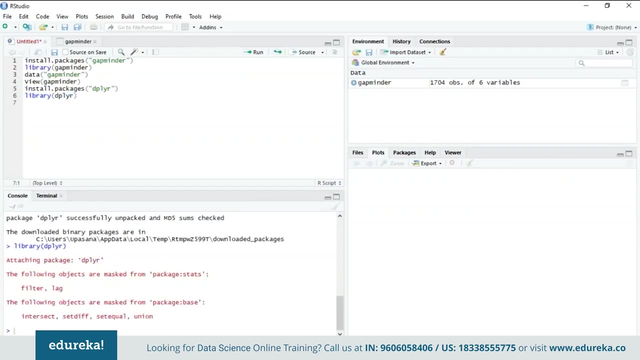 And to do that we need to use a dplyr package. So dplyr package is one of those inbuilt packages that we need to manipulate data. Let's just install this And again the library function to call it Okay, and once we've installed this, we've got access to a whole lot of sophisticated vocabulary in R. 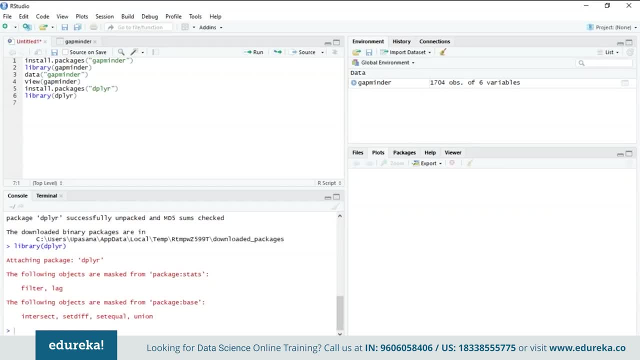 We've also got access to something called the pipe operator, which I shall explain to you about a little later in this module. So let's start by typing in And then select the country and life expectancy. So we'll be creating a data frame, but we'll do it later. 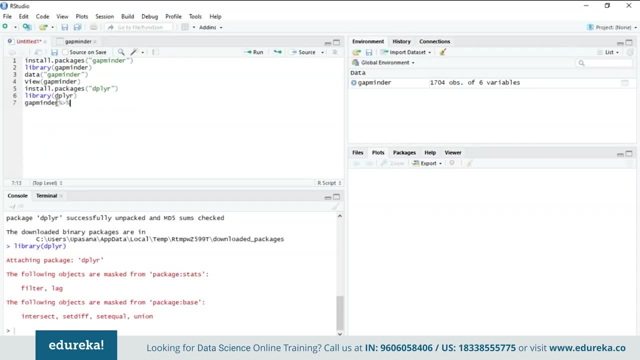 So this is what I was talking about, this percentage, arrow percentage, which is also called the pipe operator, Because, well, it looks like a pipe. Now, pipe operator lets you pipe in your data from the left into your data in the right. 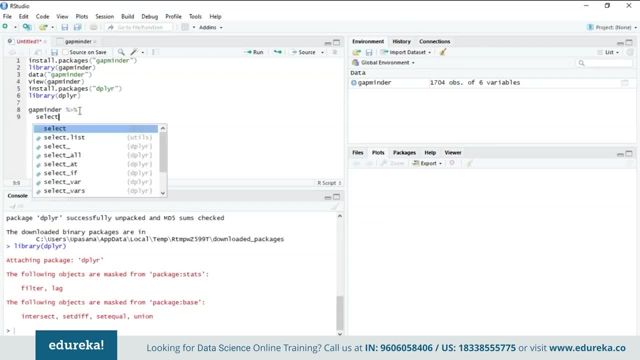 So now we're going to select the country and life expectancy And then so this is how the pipe operator is referred to, And then we will filter. In this case, we want South Africa and Ireland, So we're just going to filter these two countries. 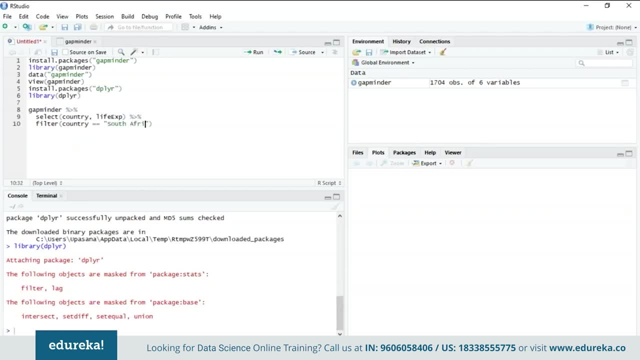 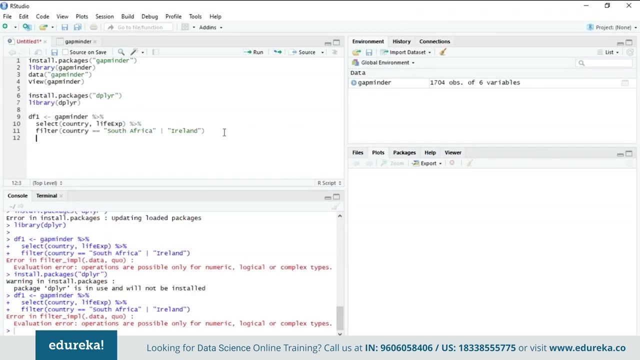 So country- South Africa or Ireland- We're going to run it, We're going to put this in a data frame, like I had mentioned before. So we want to see how the average life expectancy differs from South Africa to Ireland. Now we want to know if this difference is statistically significant or purely by chance. 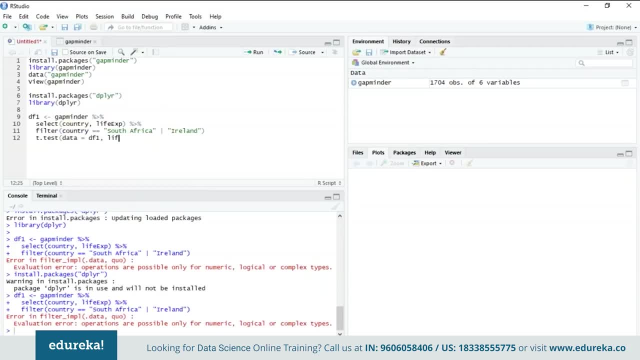 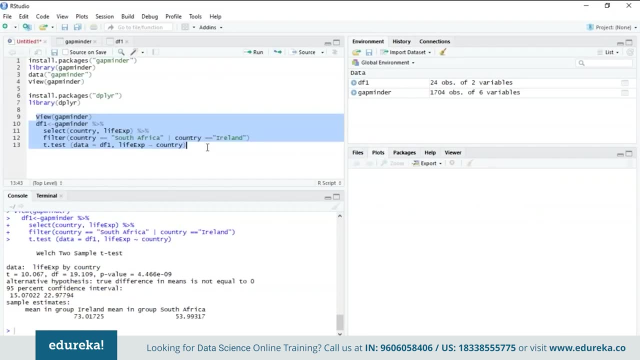 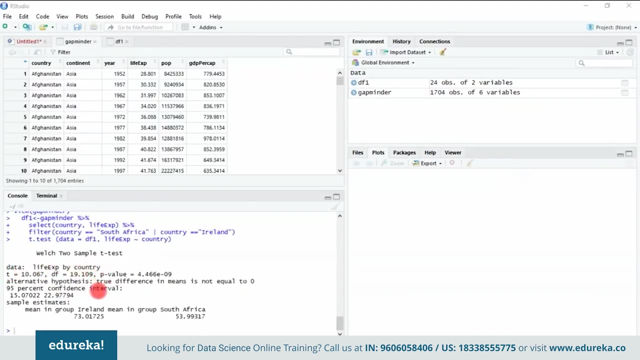 Hence we do something called a t-test. So yeah, Now apply the t-test to DF1, which is our data frame, And compare the life expectancy. We can see our results right here. So we see the mean in the group Ireland and the mean in the group South Africa. Life expectancy differs by almost 20.. 95% confidence interval lies between 15 to 22%, And 23% if we take a rounded off value. So what does this tell us, If this difference between the life expectancy is in fact zero? 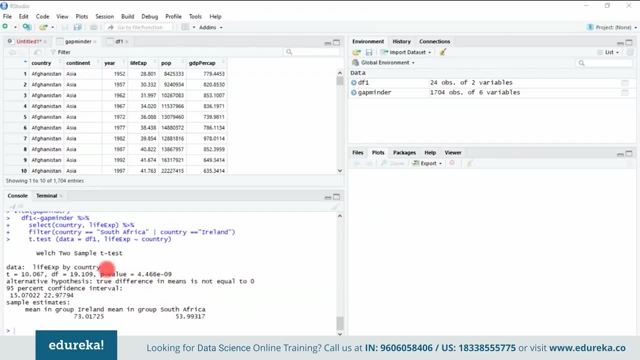 then the probability of that happening, or P, which is the probability value, which is 4.466, into e, raised to the negative of 9, which is a very, very small value- it is very, very unlikely to happen, which is almost next to impossible. 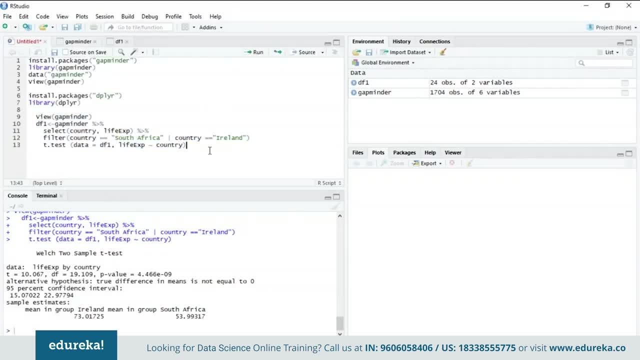 Hence it disapproves our null hypothesis. Now let's interpret this data using the ggplot2.. Again, we shall install the package and tell R that we want to use it. Now we're just going to type gapminder. 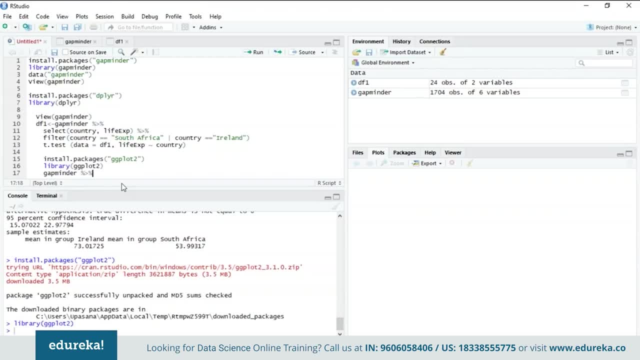 And then now I'm just doing this to show you how much control the pipe operator can give you. Now we want to specify the aesthetics and filter by GDP per capita. Filter by GDP: It automatically comes over. GDP per capita less than. 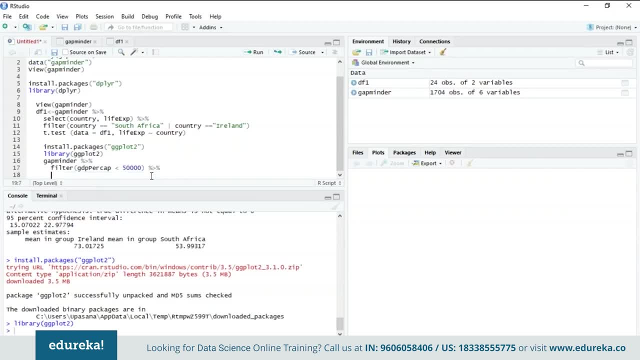 50,000.. And then we'll be specifying the aesthetics of the plot. So AES X is equal to GDP per capita, Y is equal to life expectancy. Now we want to specify the aesthetics. We want the life expectancy to map out against Y axis. 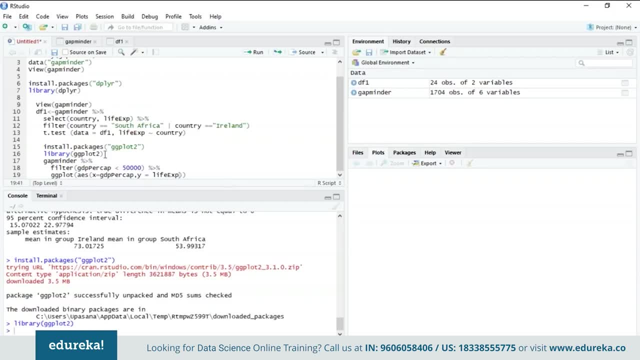 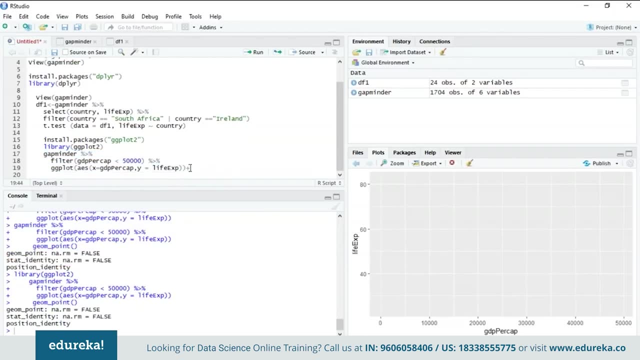 and the GDP per capita to map out against X axis. So let's just run the code and see: Okay, So we use the plus sign to see what geometry needs to be used on the canvas. So I'll be using this, the geometry point. 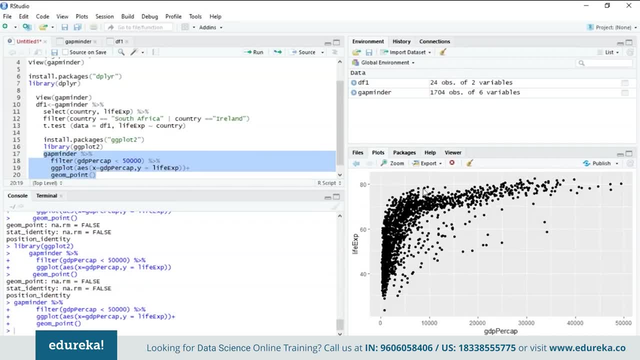 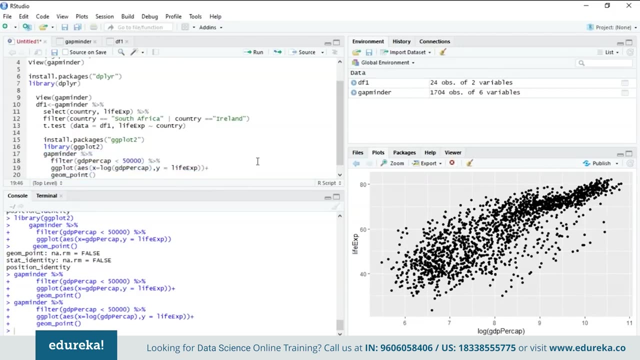 Let's run this and see We get a basic scatterplot. To get a better graph, let's just do a log transformation of our GDP per capita and run this Much better. Now this looks a little bit busy, So let's just color all the dots by continent. 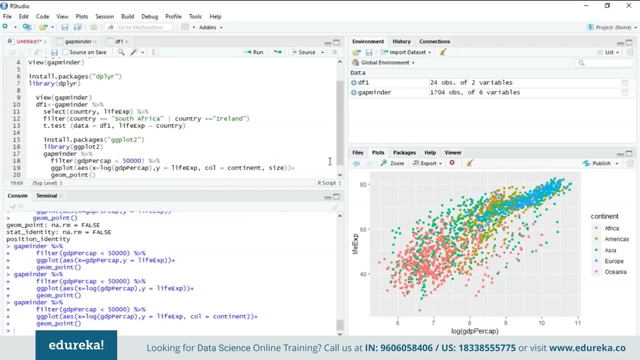 And we can also change the size of each bubble by the population size. There you go. Looks very busy, Looks very opaque. So let's just make these bubbles a little transparent. All we have to do is type alpha equals 0.6.. 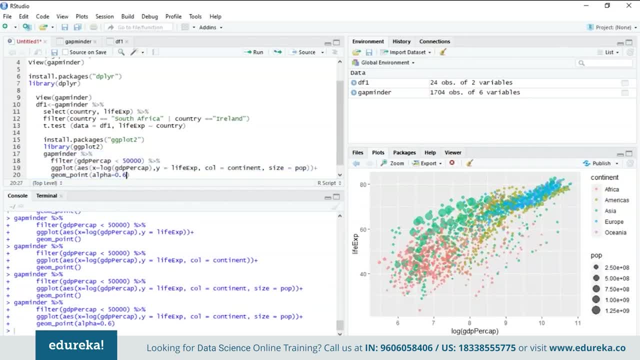 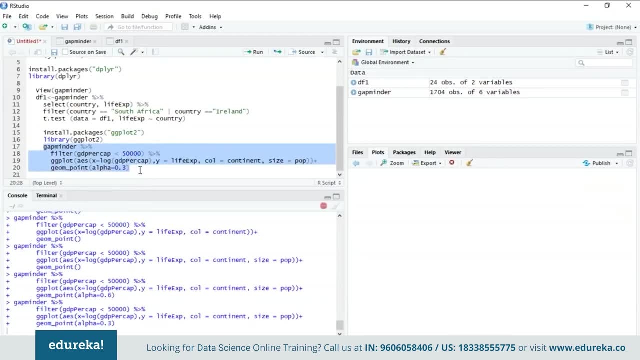 Okay, slightly better, Let's try 0.3.. By trial and error you can basically see the kind of transparency you want. Okay, this works for me much better. Now, if we want a smooth, a linear graph, we can just add QM smooth. 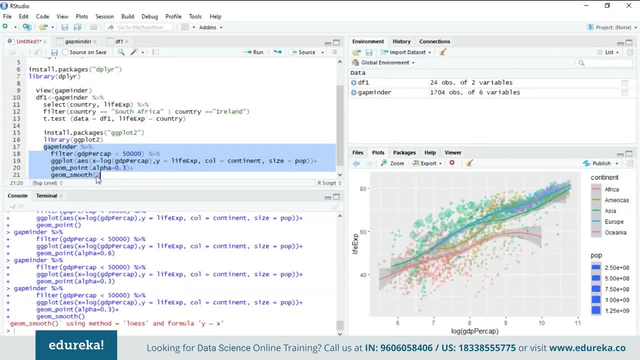 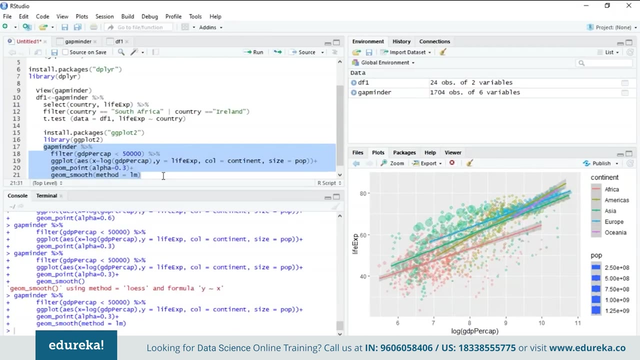 Let's see what that does. Yeah, it gives us lines showing a pattern or a trend in the bubbles. If you want a more, more linear method, all you can do is type method equals LM. We have straighter lines Now. it still looks very busy to me. 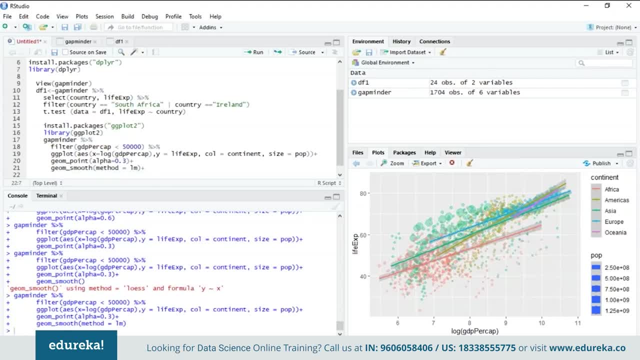 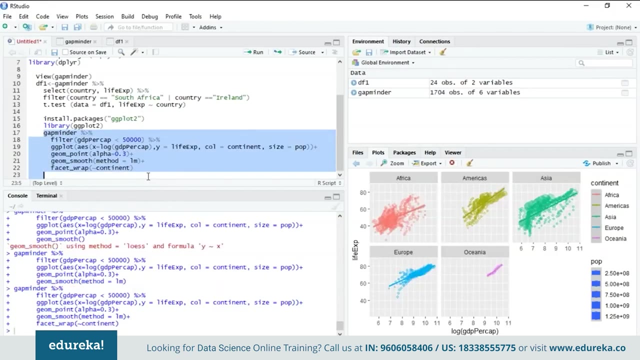 So I am just going to separate it, continent wise, into different graphs. So facet, there's something called as facet wrap And I'm going to type continent. Now that we have five different graphs, we're going to have five different graphs for different continents. 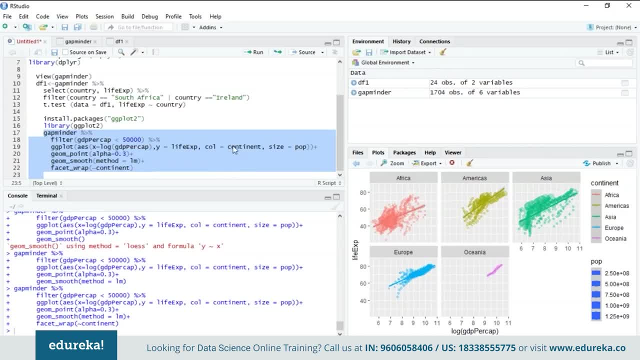 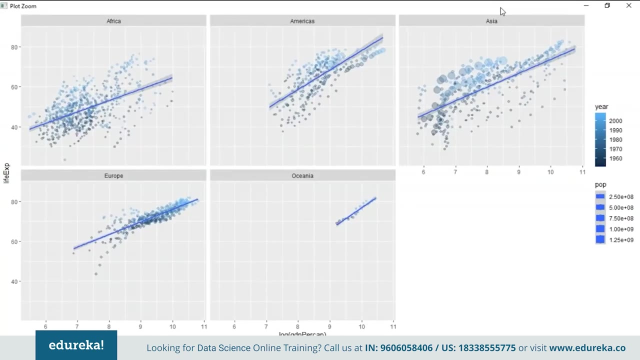 I think segregating them by color is not required, So let's just color this by year, shall we? Now, if I zoom this, if I zoom the plot, you see that now we have one graphic which has life expectancy GDP per capita population size. 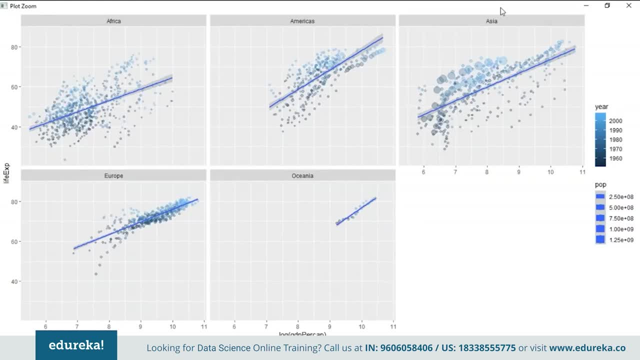 by continent and date. Okay, Five variables in one graphic. that doesn't look too busy or messy, And this is what R has to offer. Hence, it is completely a statistician's programming language. With that I conclude my session on statistics for data science. 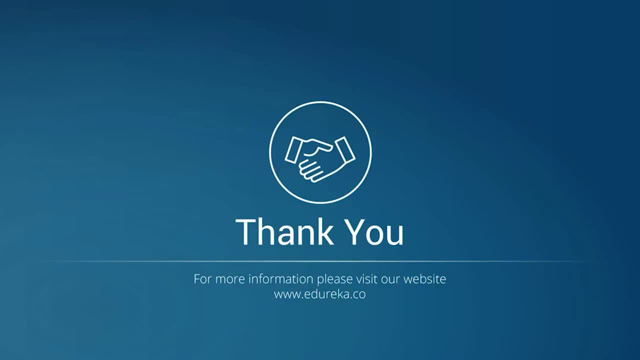 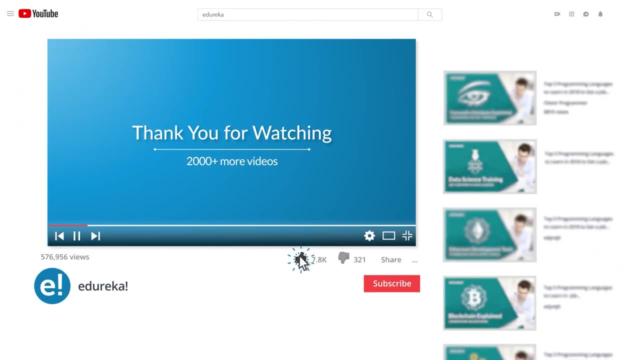 If you have any queries, feel free to leave them in the comment section below. Thank you, and have a great day ahead. I hope you have enjoyed listening to this video. Please be kind enough to like it and you can comment any of your doubts and queries and we will reply them to you. 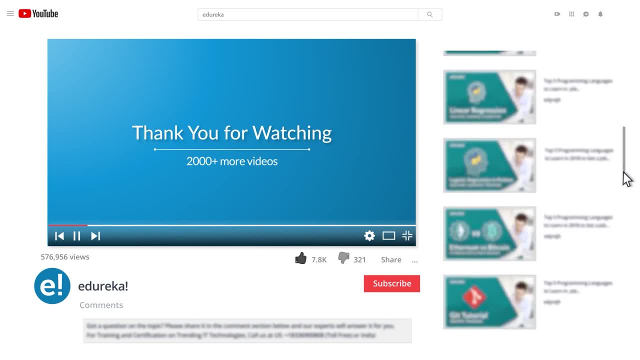 Do look out for more videos in our playlist and subscribe to Edureka channel to learn more Happy learning. 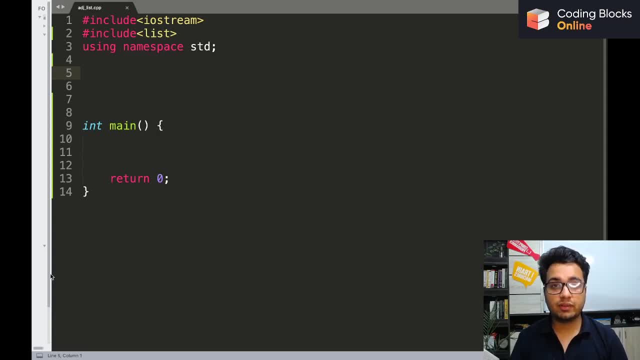 Hey guys, so now you have understood what a graph is. So it's time to implement our first graph data structure using a adjacency list. So let's begin. Okay, so let's say: this is the graph that is given to us And this is how the adjacency list representation of 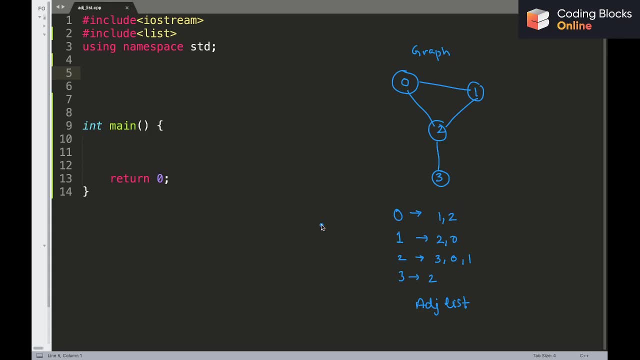 this graph would look like, And now there can be multiple ways to store this graph, So we may use a hash map that we will see in the next video. But just to make the implementation simpler, and since we have nodes which are numbered from zero to n minus one, okay so,